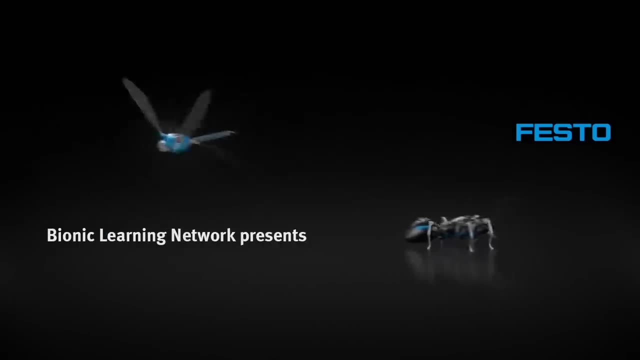 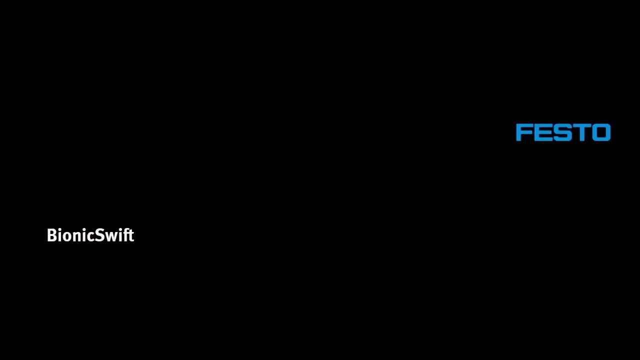 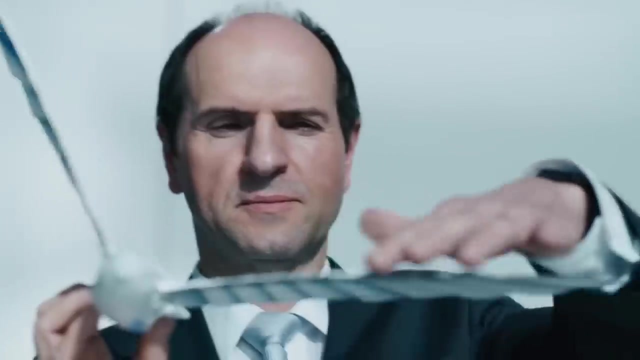 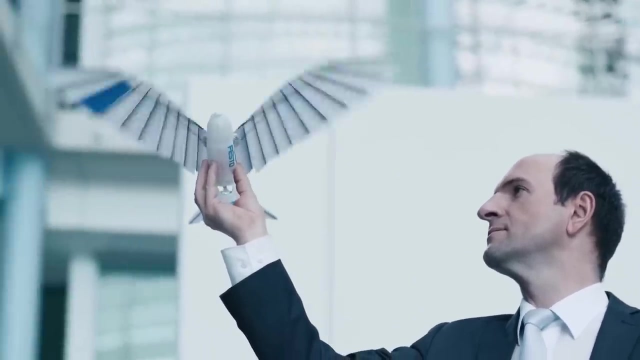 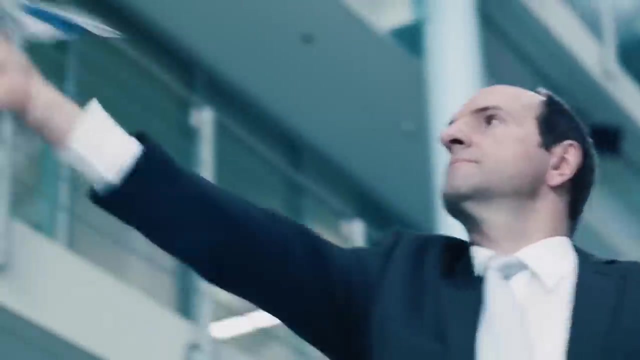 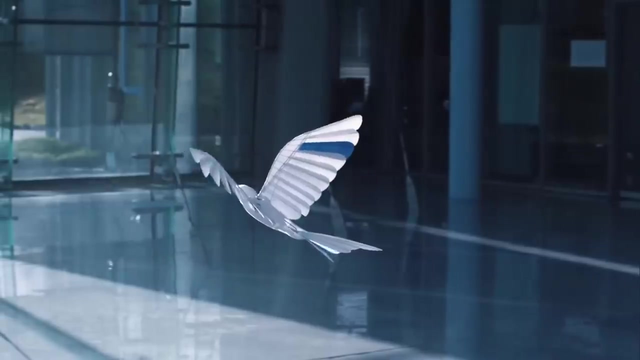 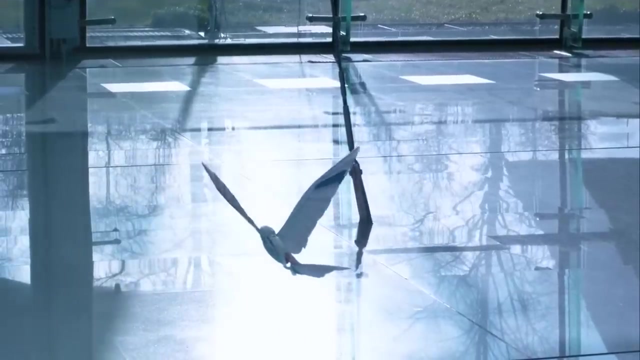 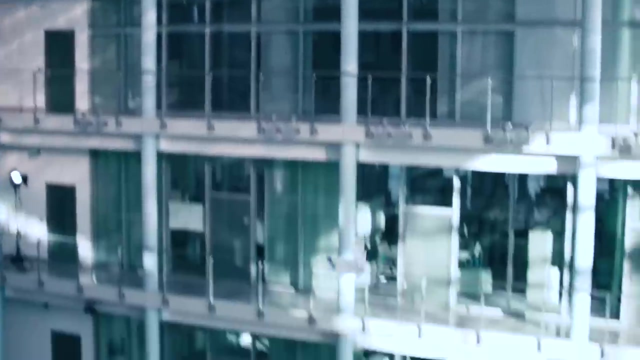 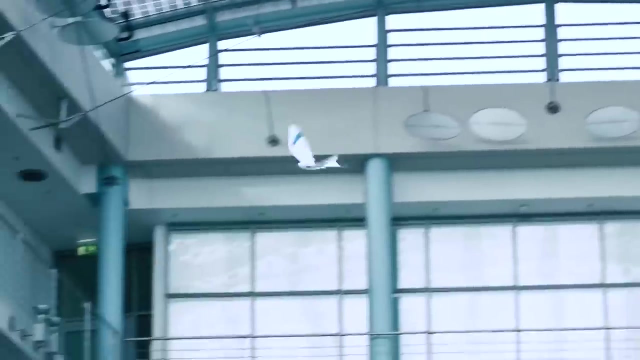 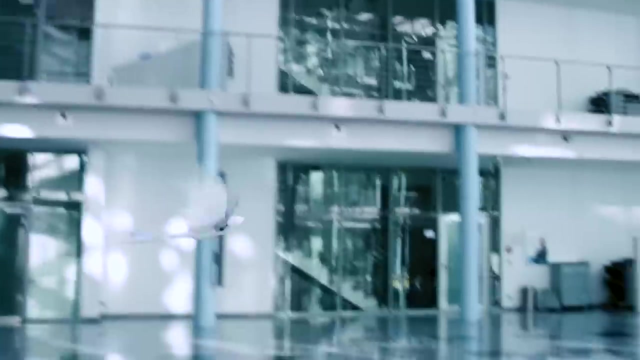 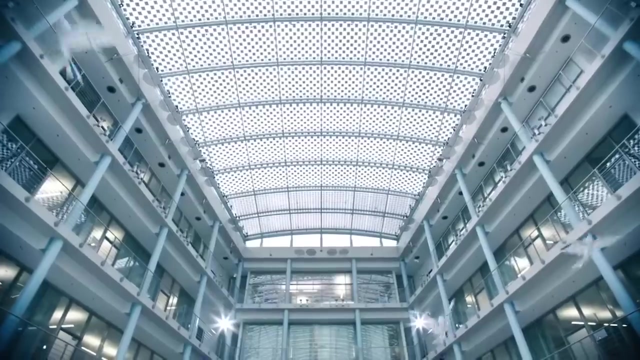 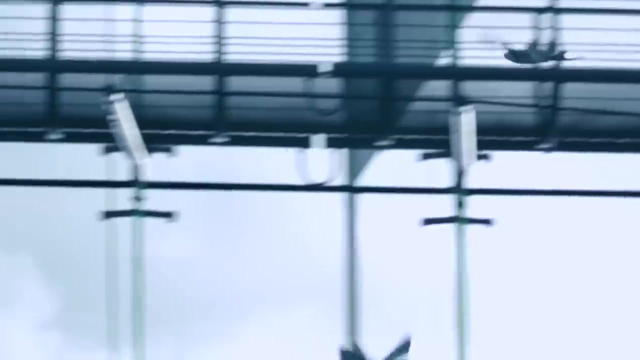 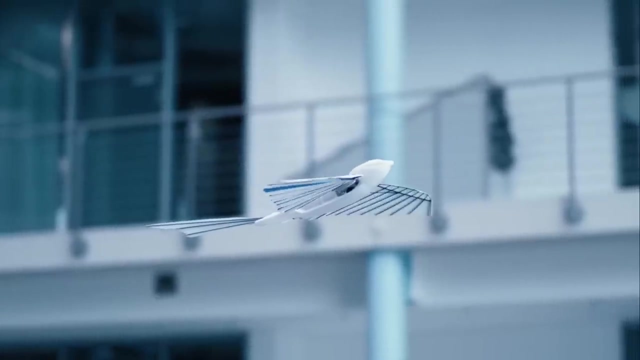 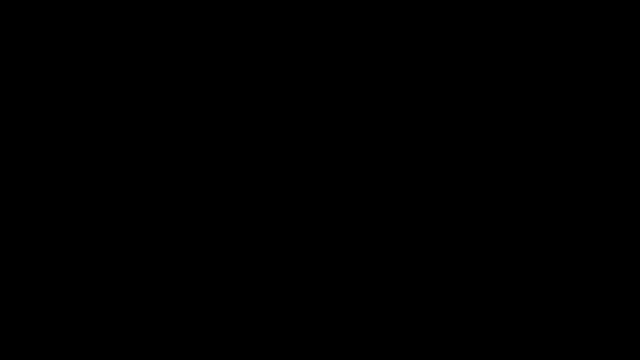 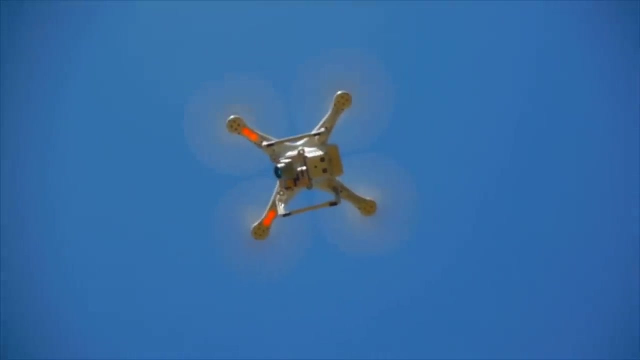 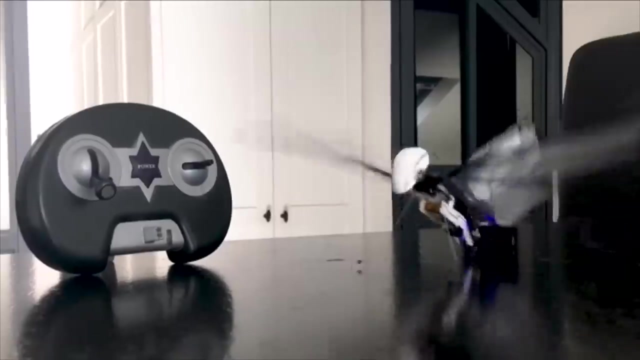 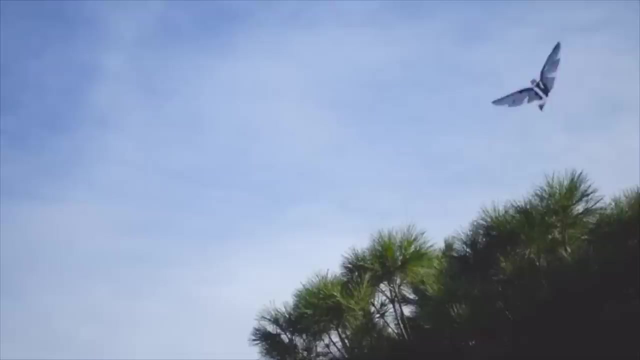 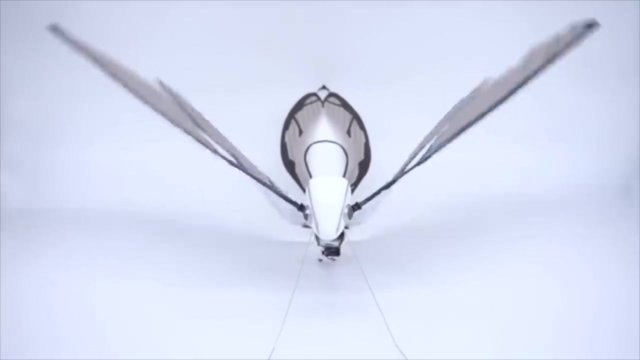 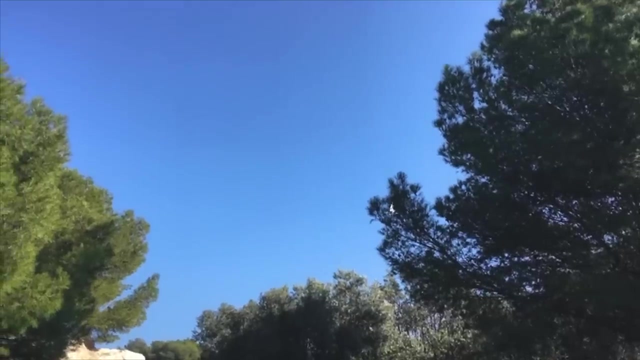 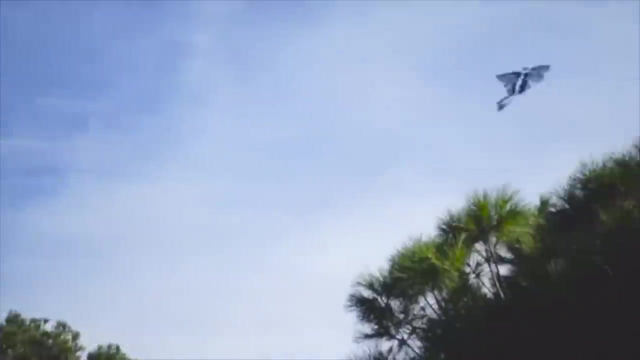 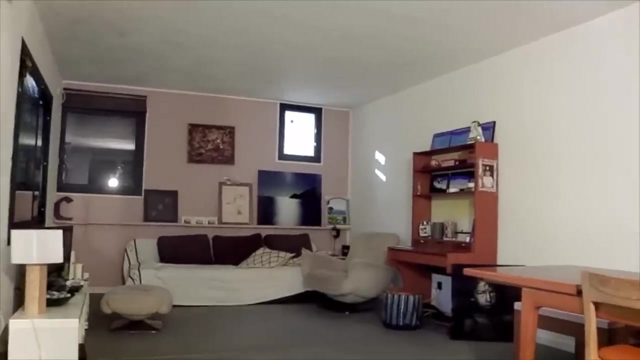 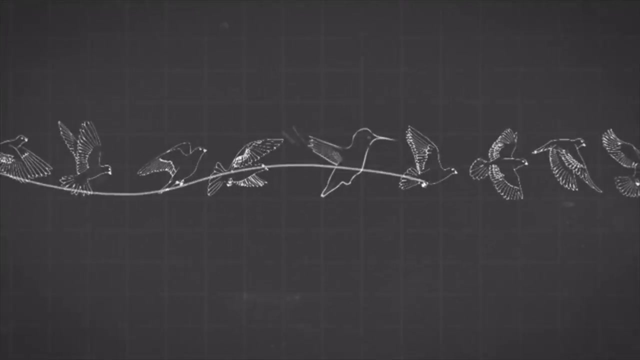 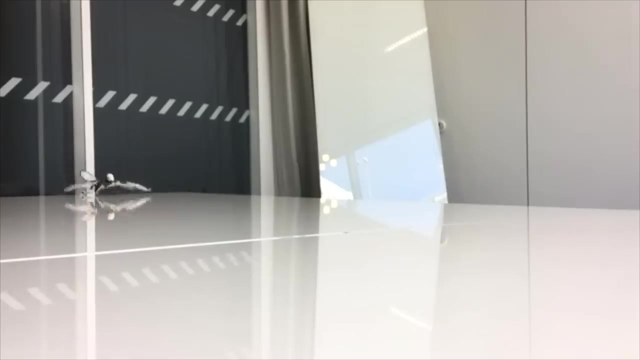 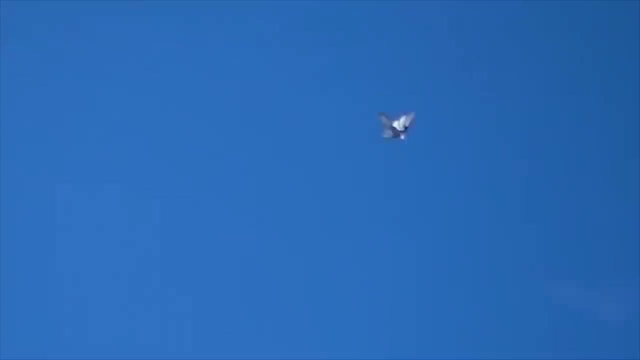 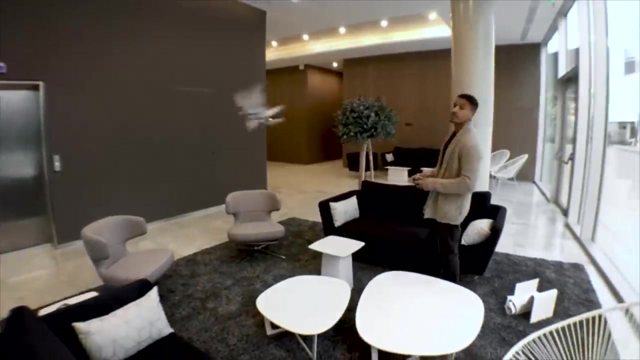 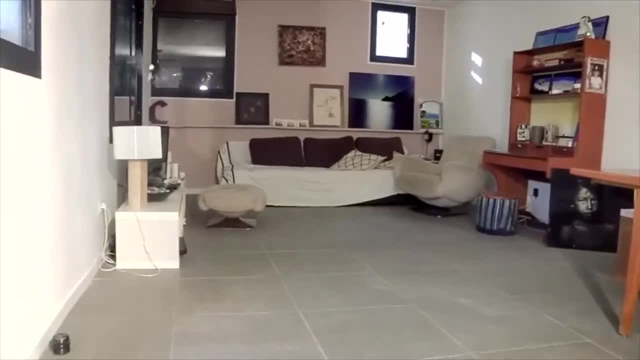 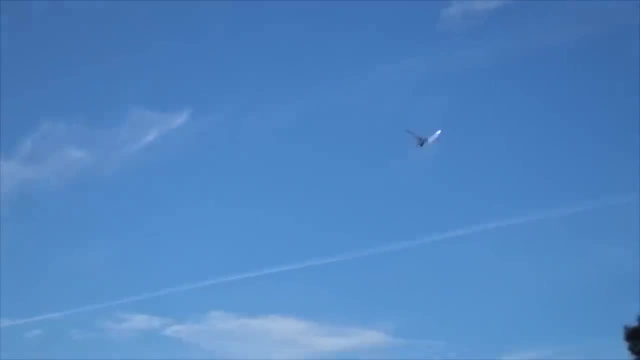 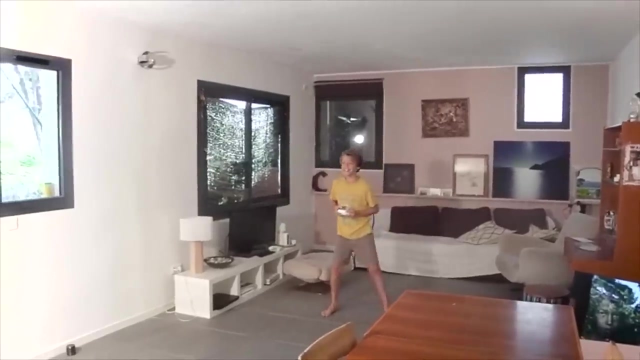 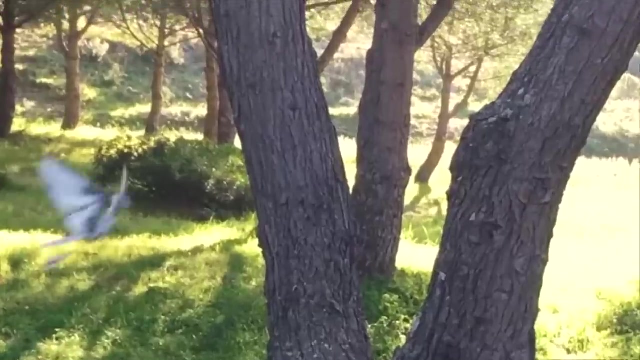 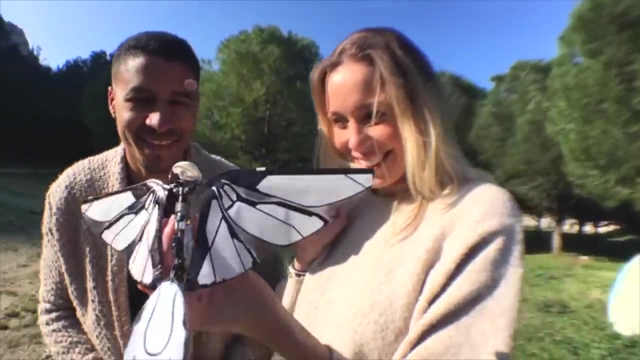 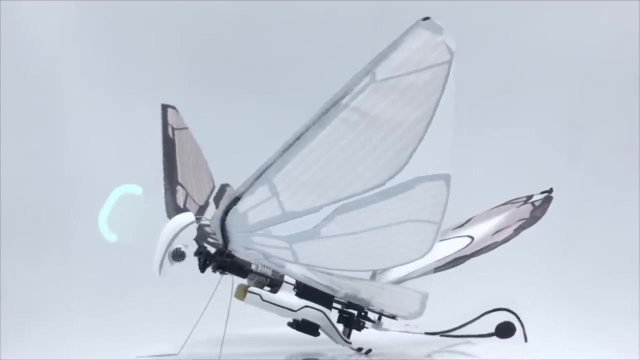 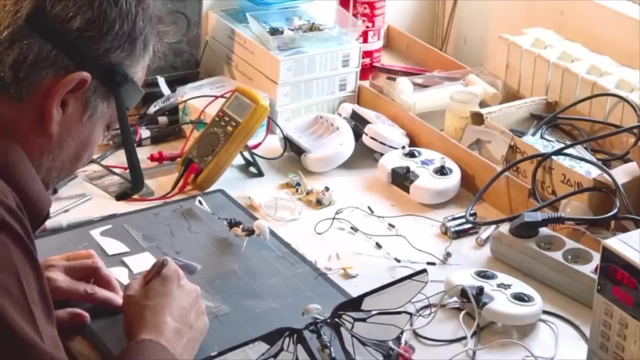 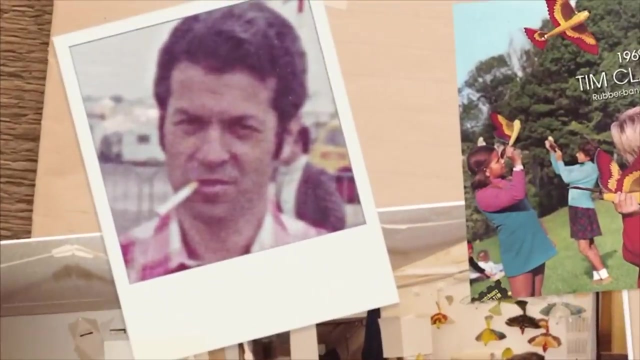 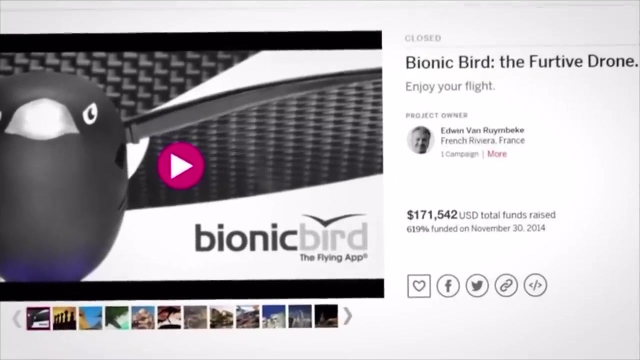 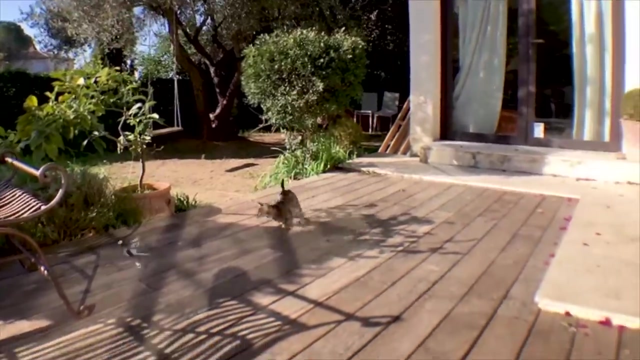 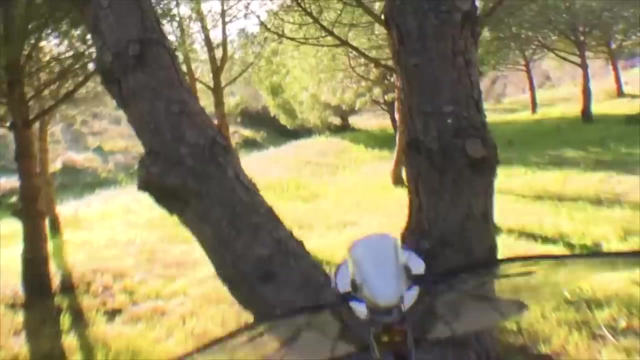 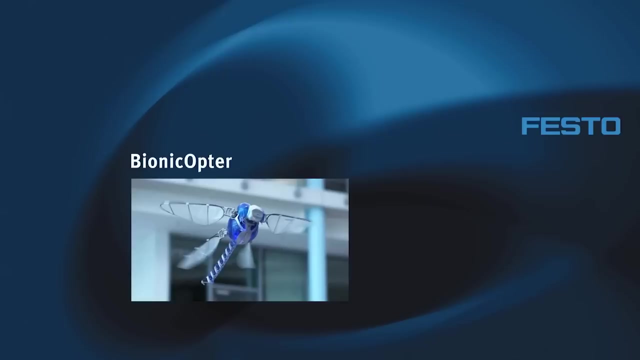 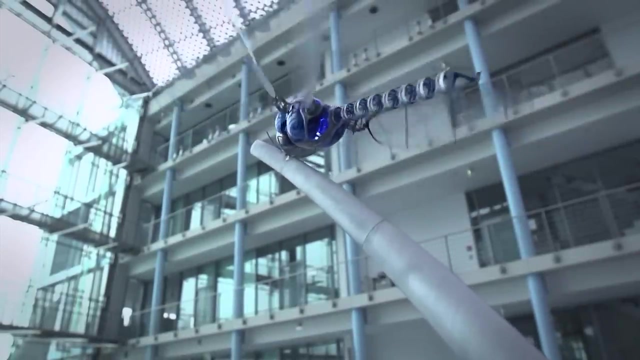 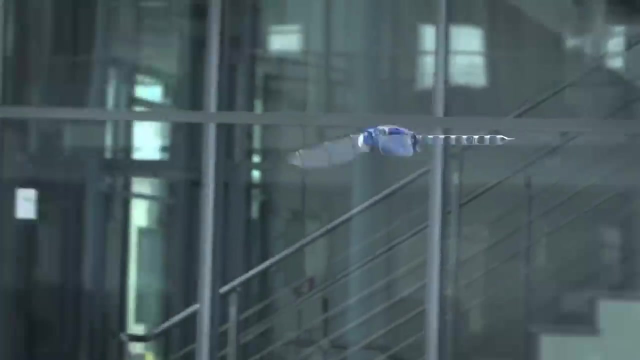 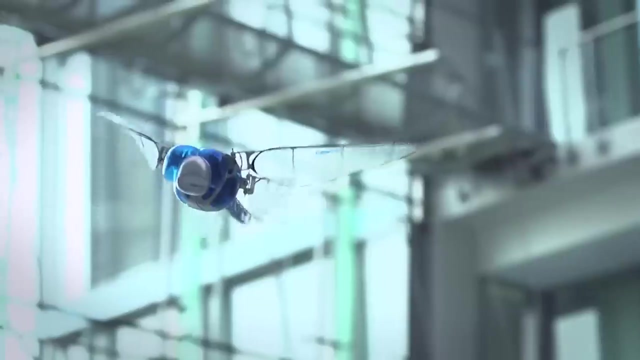 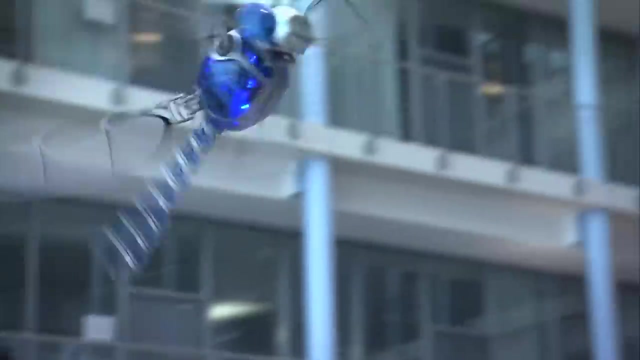 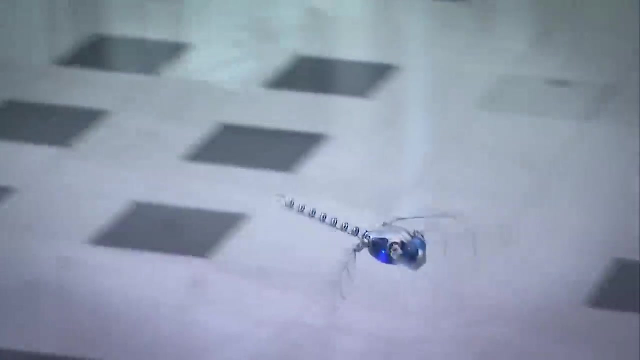 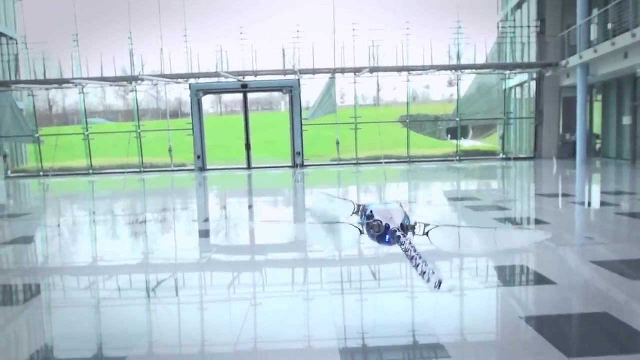 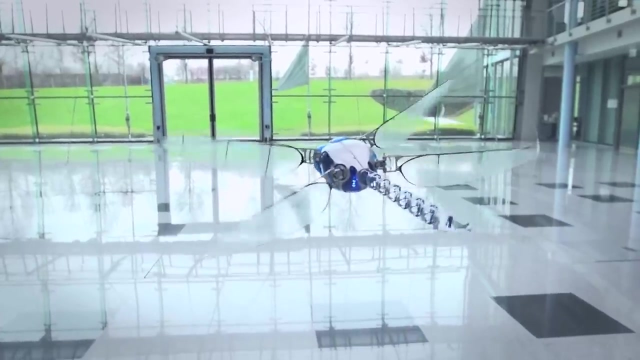 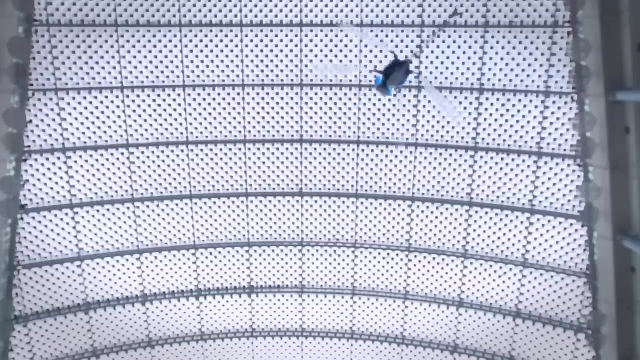 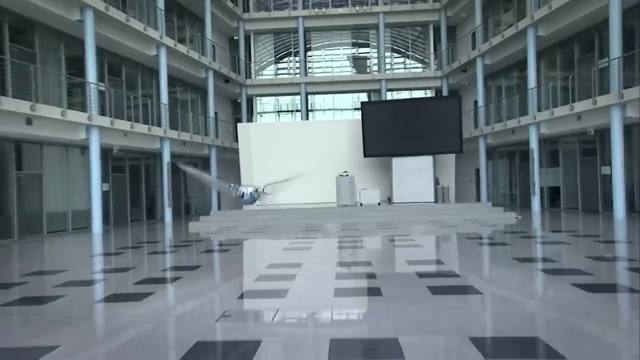 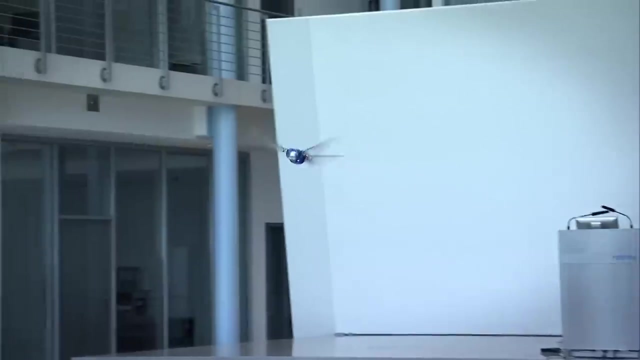 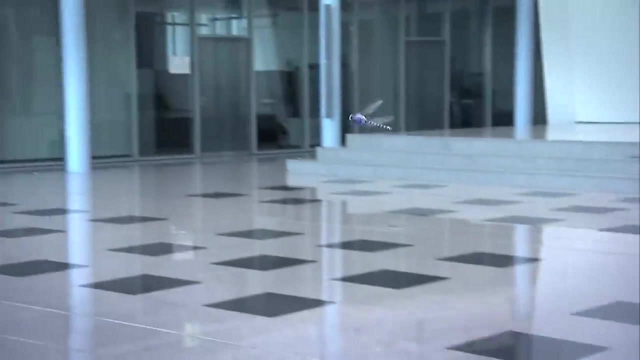 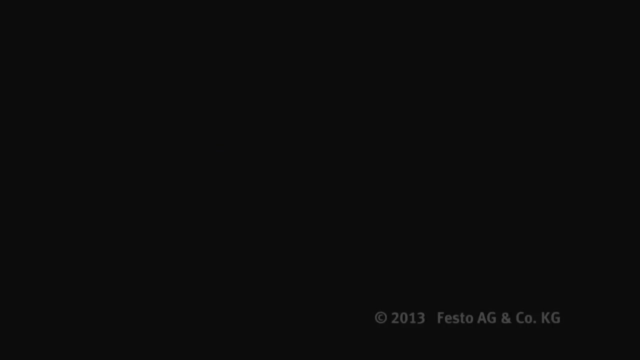 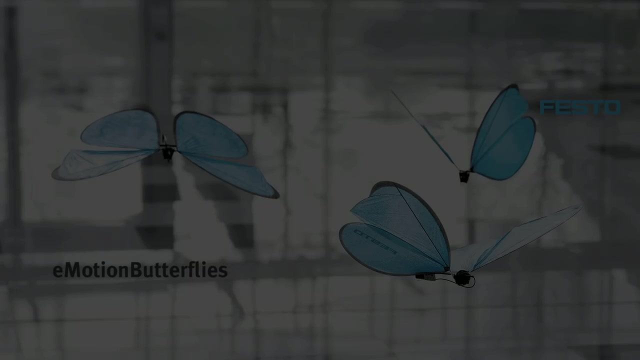 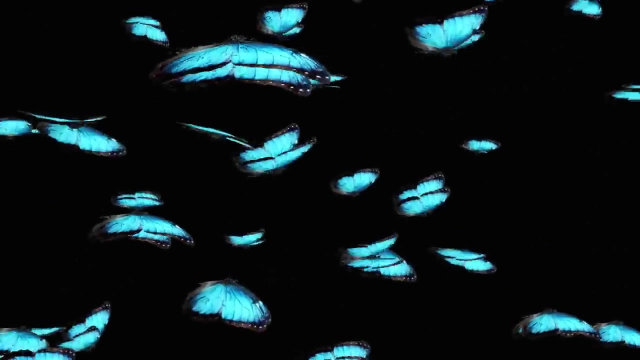 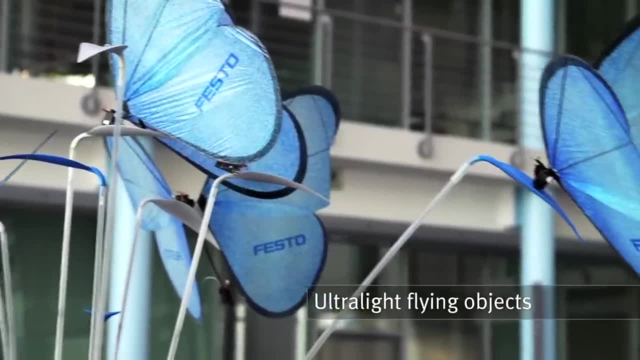 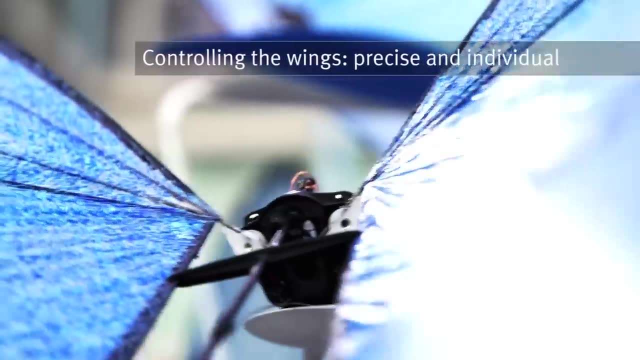 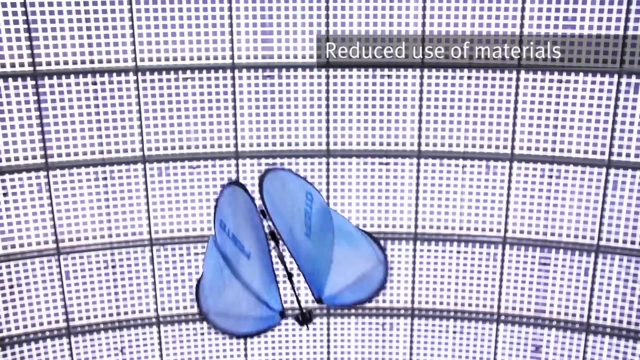 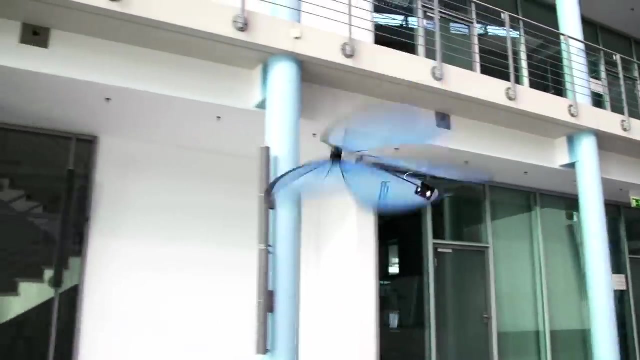 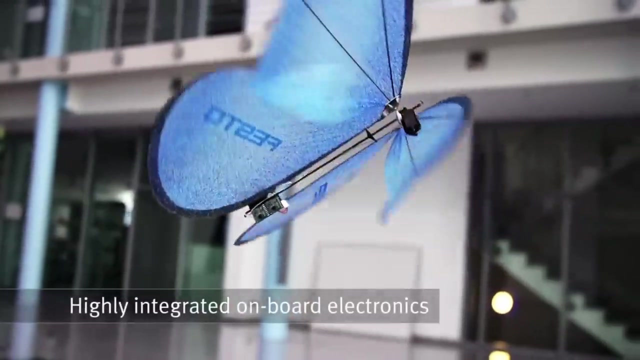 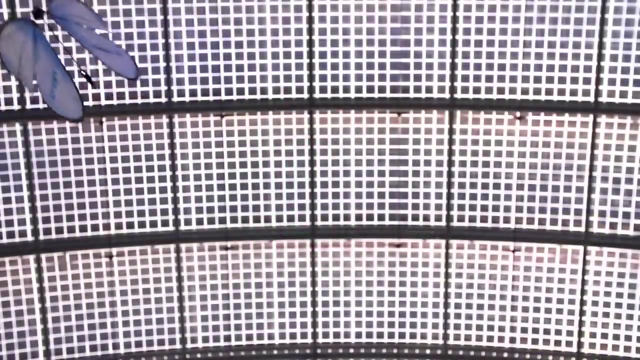 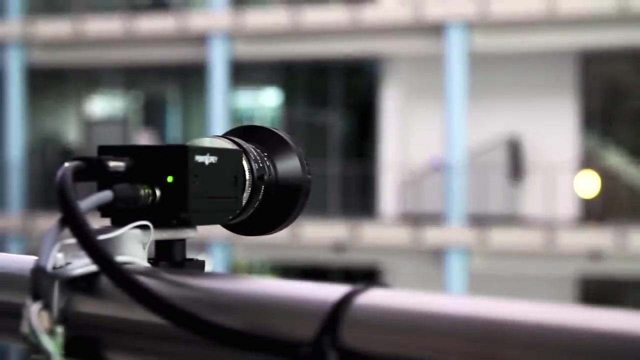 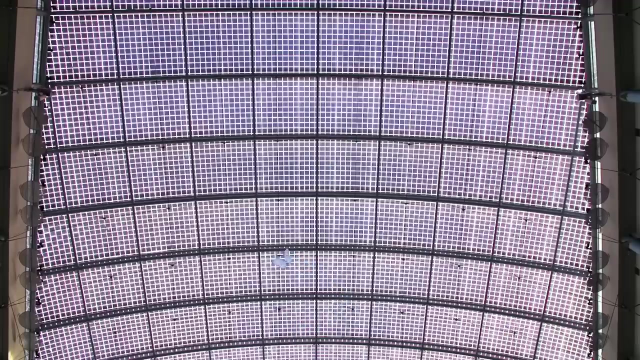 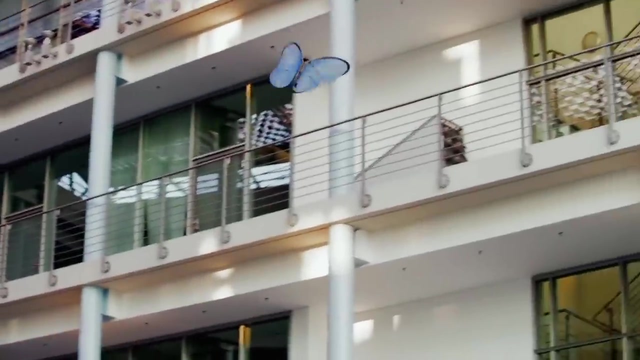 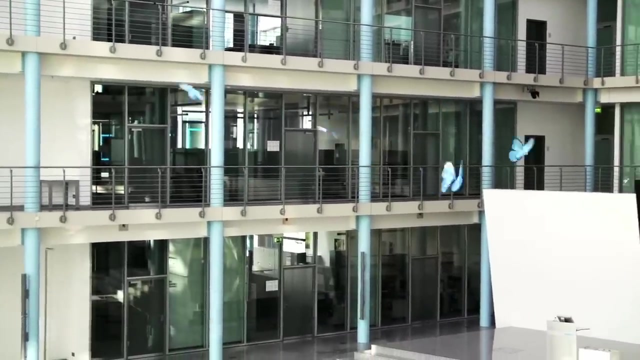 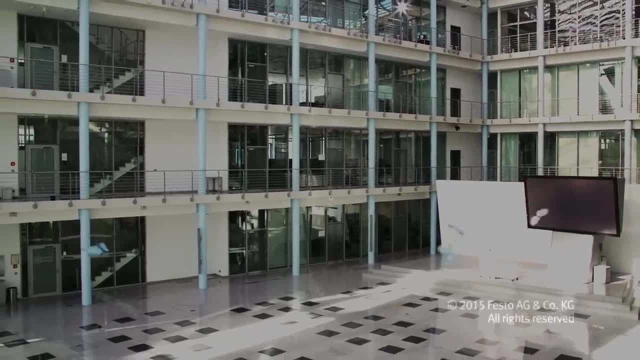 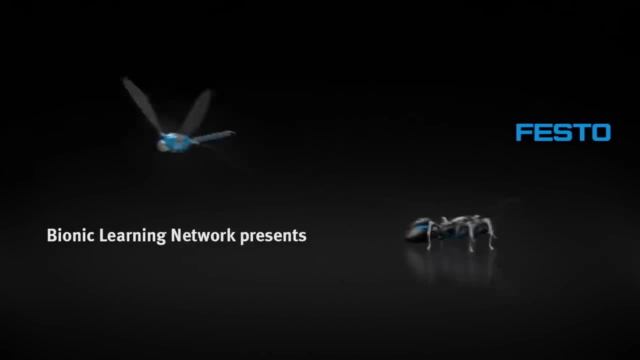 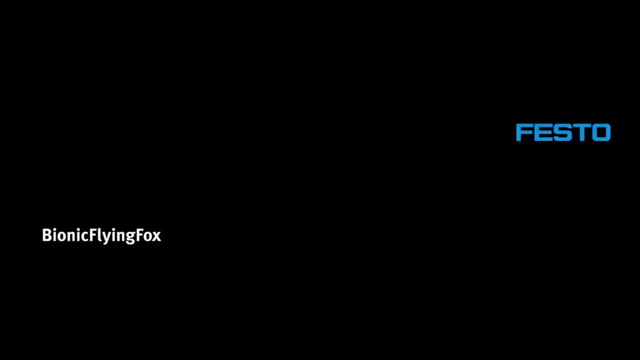 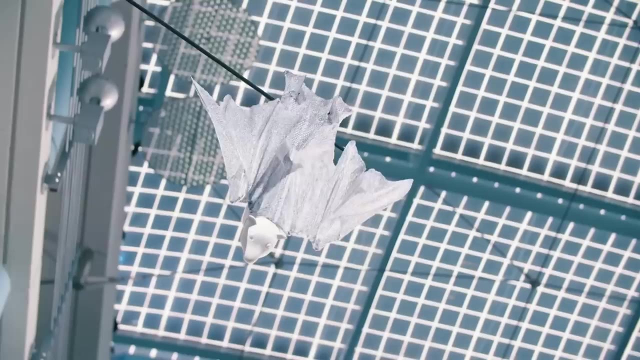 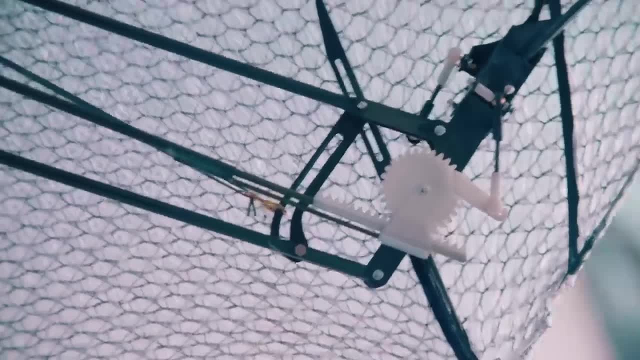 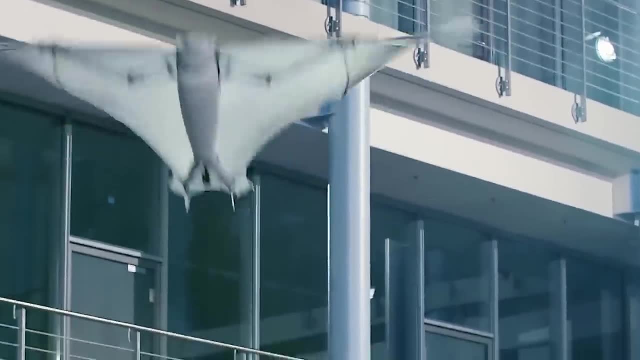 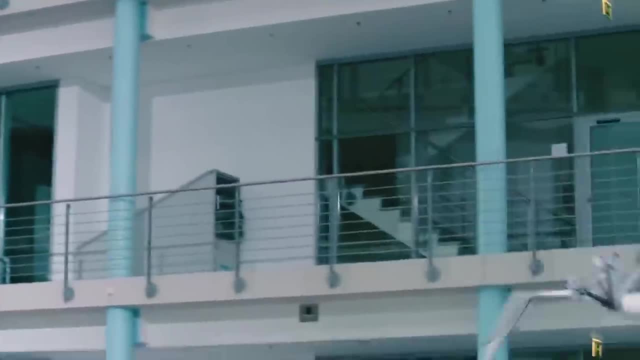 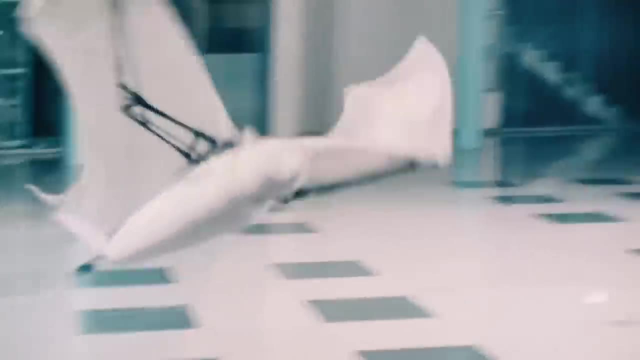 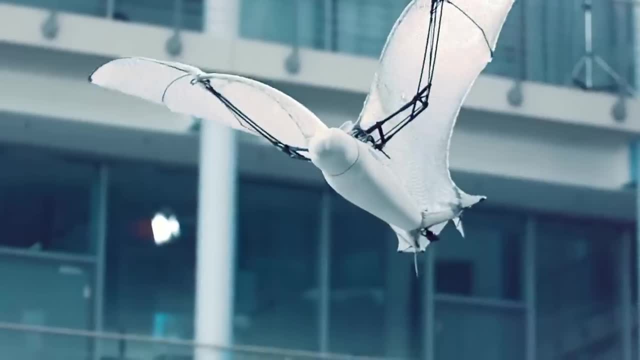 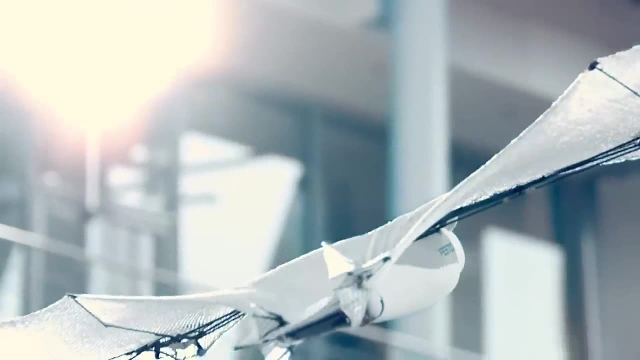 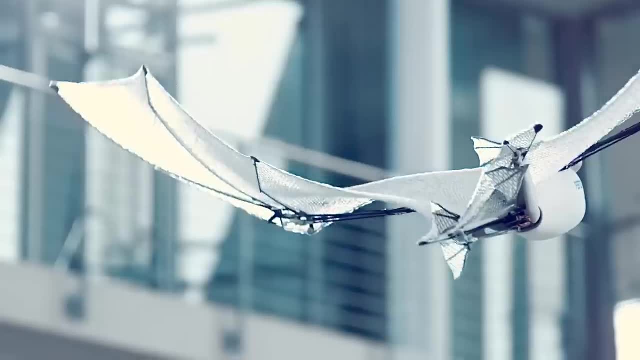 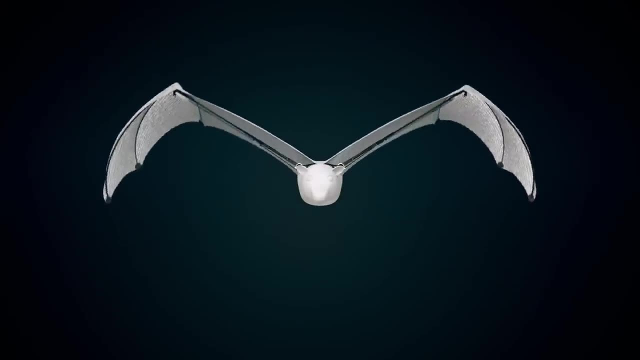 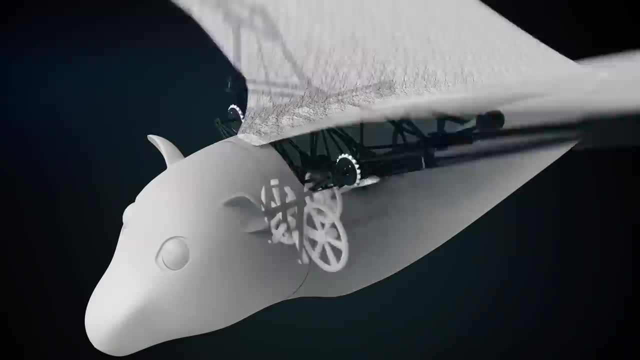 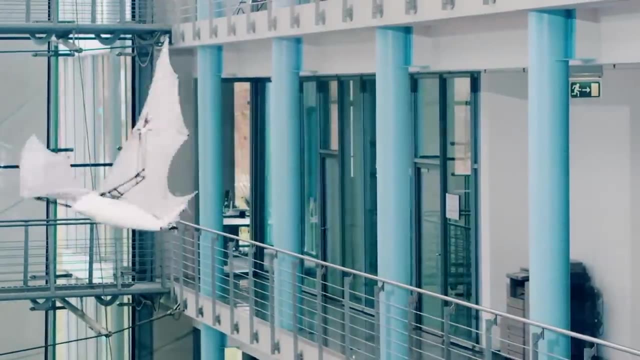 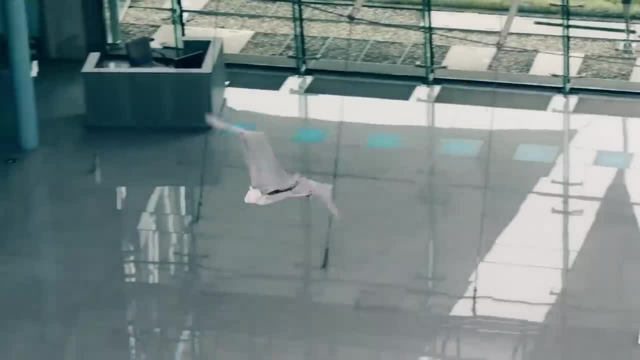 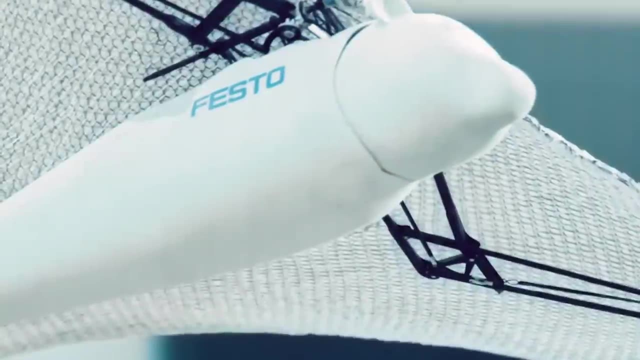 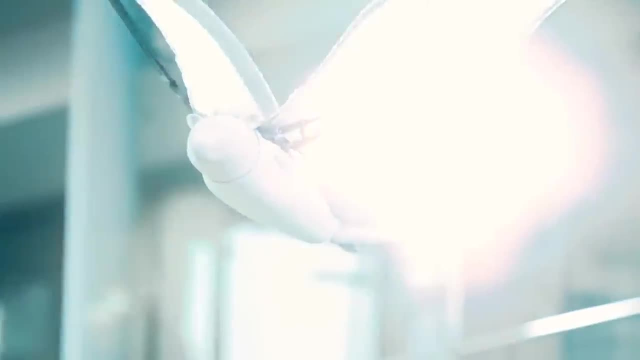 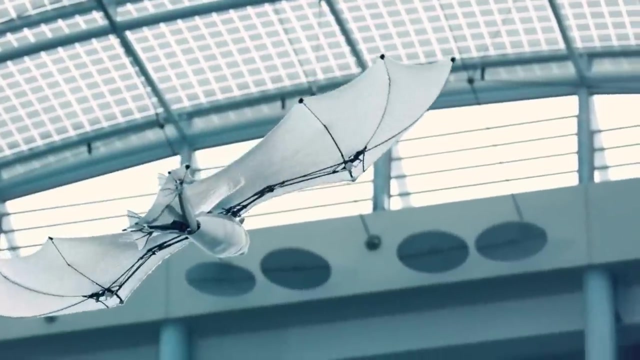 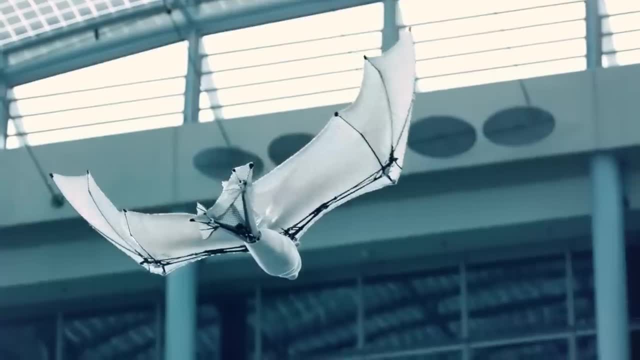 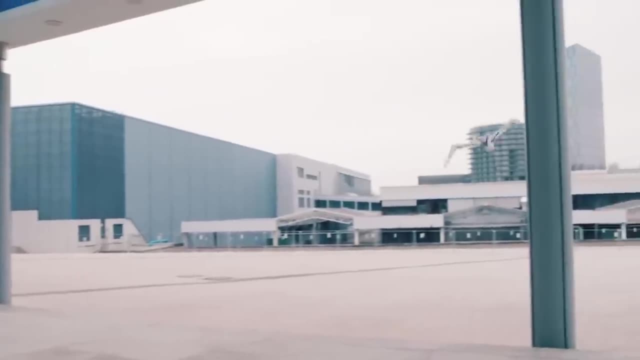 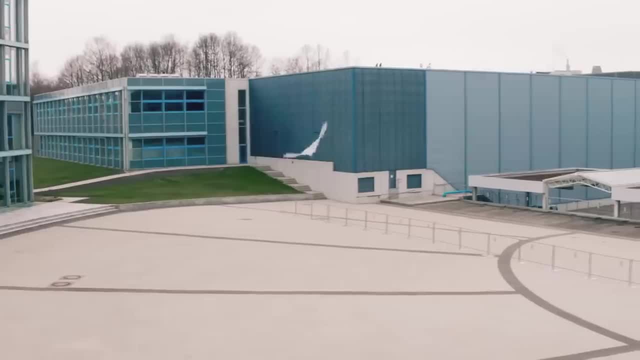 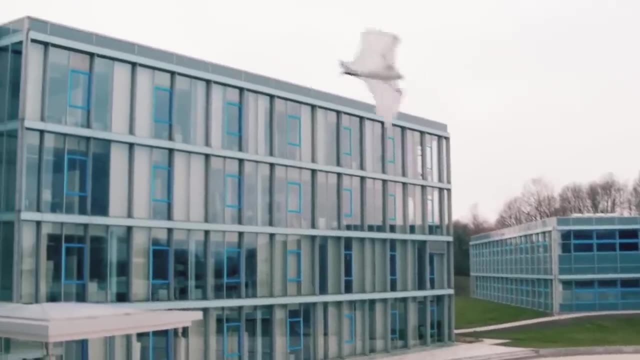 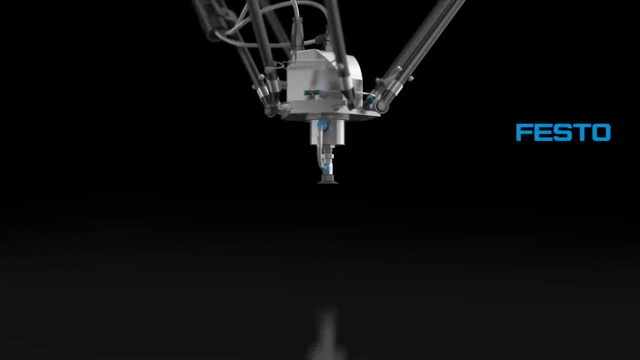 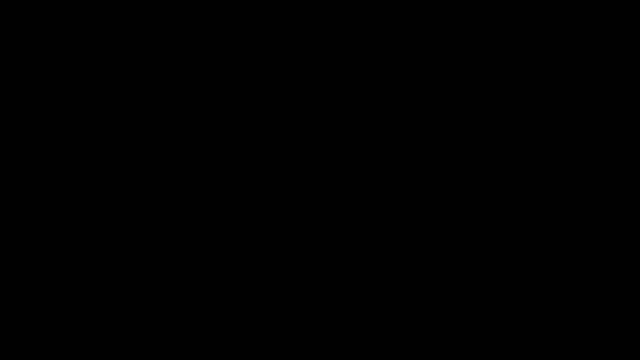 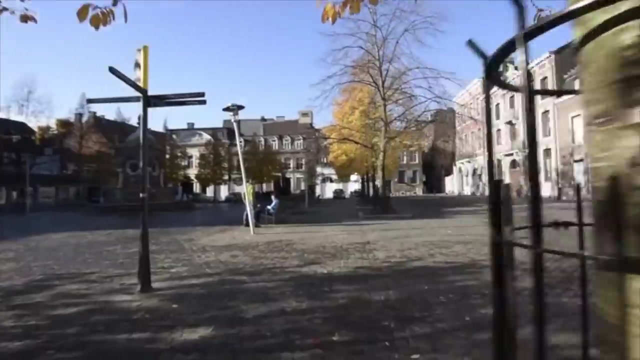 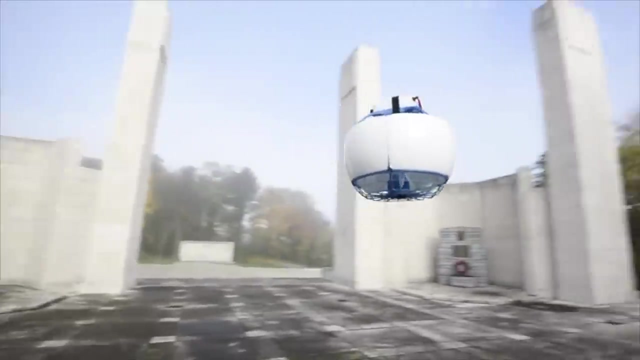 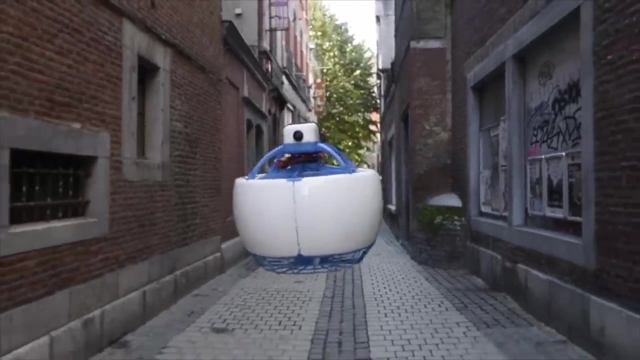 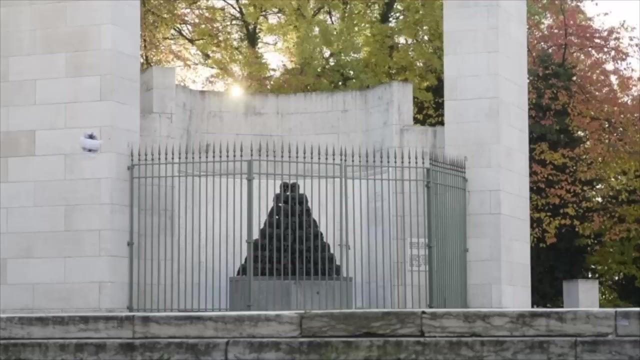 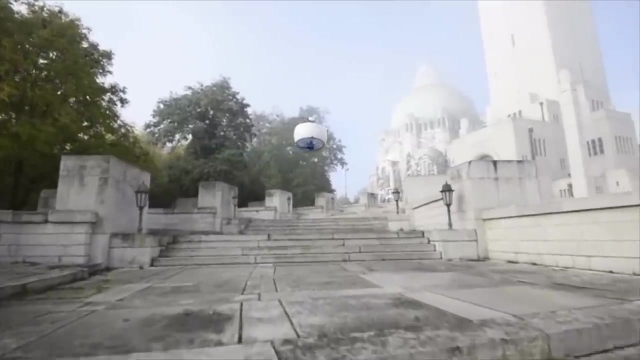 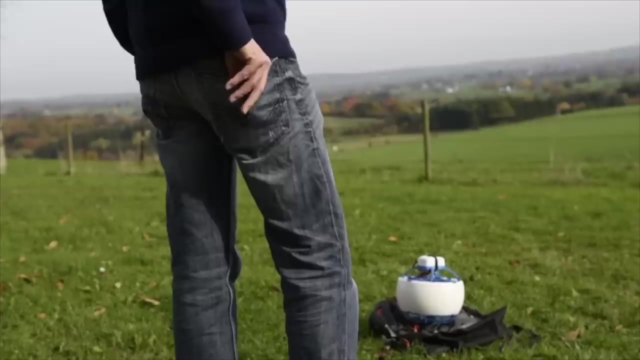 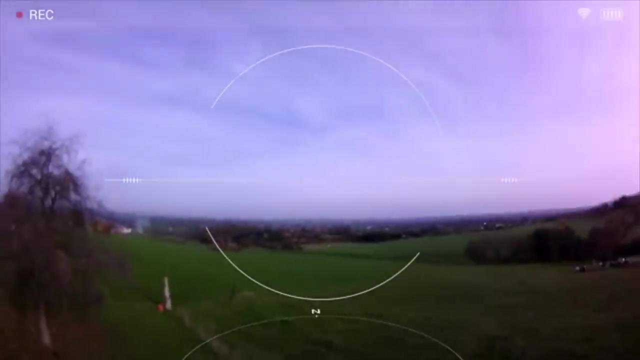 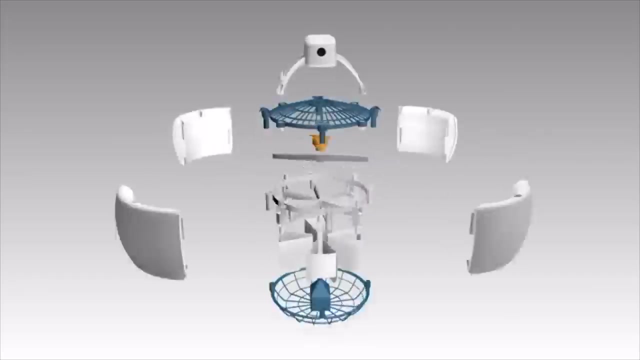 Transcription by ESO, Translation by: —. Transcription by ESO, Translation by: —. Transcription by ESO, Translation by: —. Thanks for watching. Thank you for watching. It's made of a single-shifted propeller and four control vanes for stability. 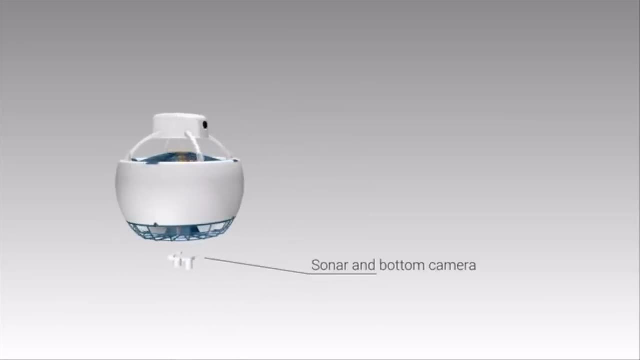 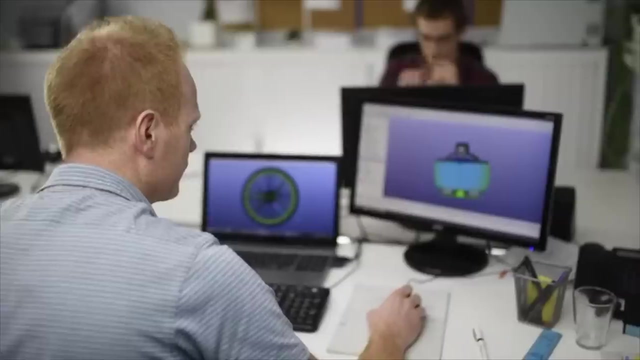 It has the same size and weight of a soccer ball. It's packed with sensor, a powerful onboard computer, an HD camera and a Wi-Fi connection. We wanted Fly to be smart and autonomous, so you don't have to be always piloting it. 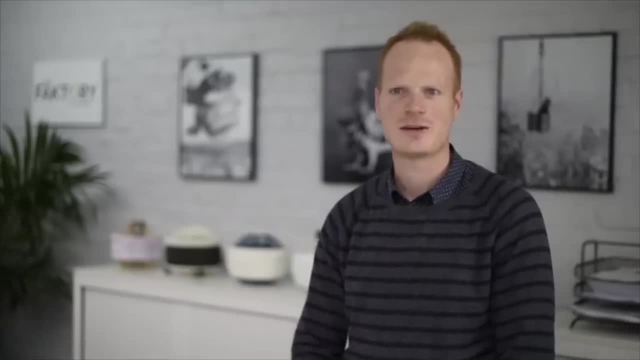 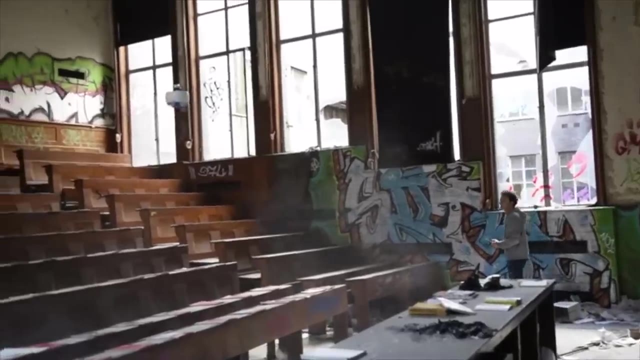 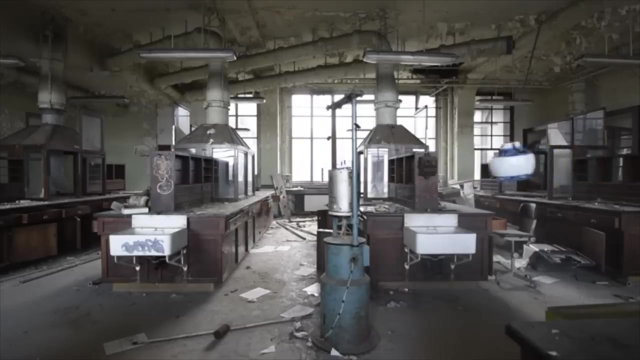 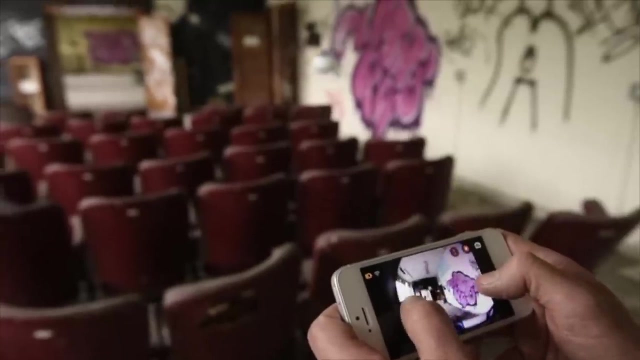 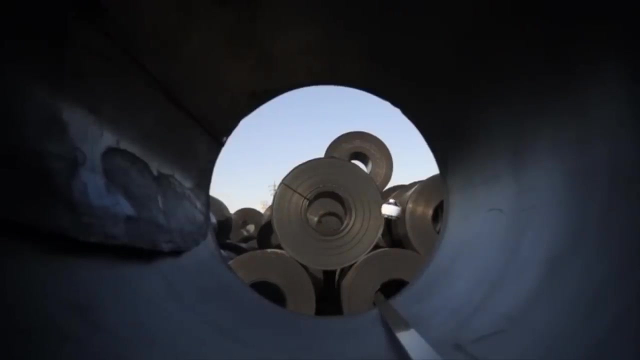 You can select a simple mission through the mobile app and just enjoy the live streaming. Fly is a lot of fun to play and interact with, But it's more than a toy. It's really a platform on which you invent the future of flying robots.